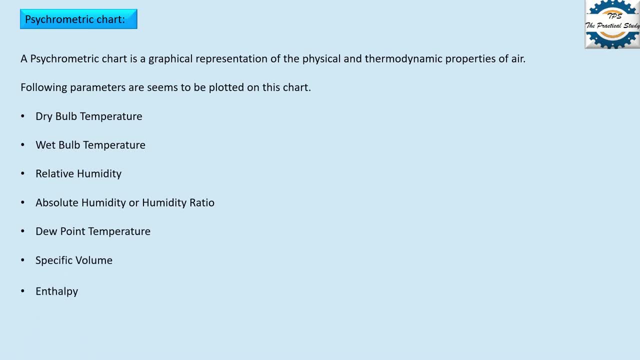 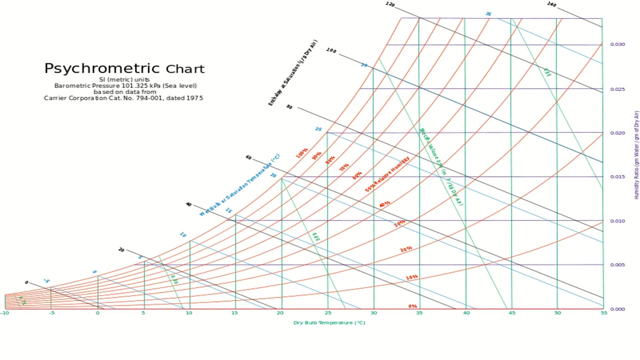 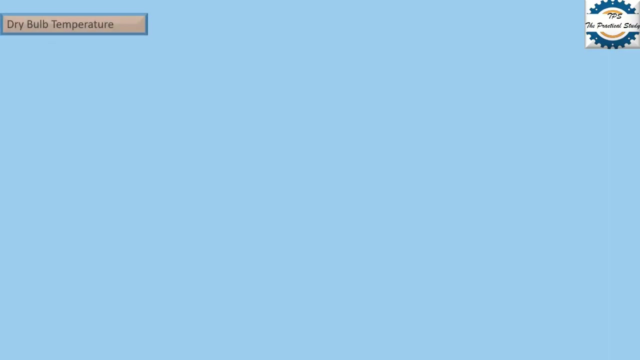 dew point, temperature, specific volume and enthalpy. You will learn all these parameters one by one and plot it on psychometric chart. This is psychometric chart and I am not going to discuss it right now because it seems to be very complex. Let's make it simplest, step wise. First of all, we will discuss dry bulb temperature. 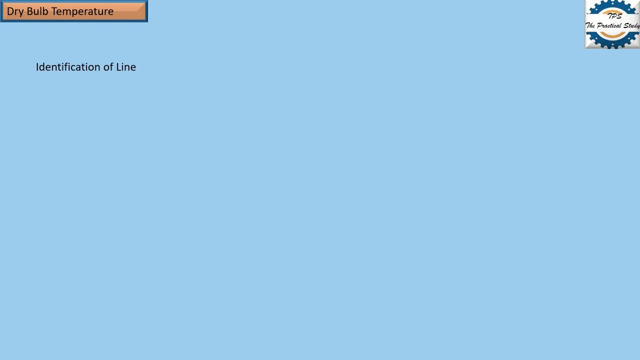 If dry bulb temperature is greater than standard temperature or it is below the standard temperature, then we know that the temperature can be measured by a normal thermometer. For better understanding of psychometric chart, two points should be kept in mind. Number one: you need to identify the line that which line represents which parameter and where. 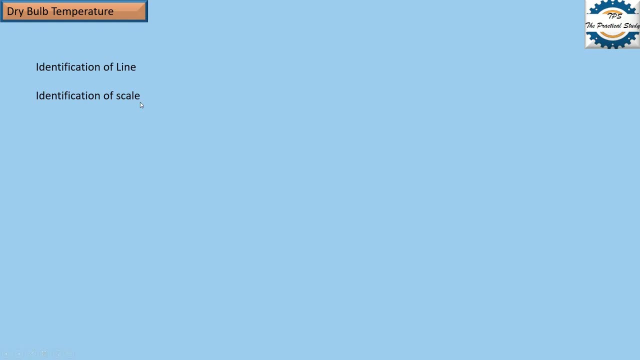 is the scale of parameter. If you keep in mind these two points, then you can understand what is the scale of parameter. So what is the scale of the parameter right now? If you know these two, if you keep in mind these two points, then you will learn these two points. 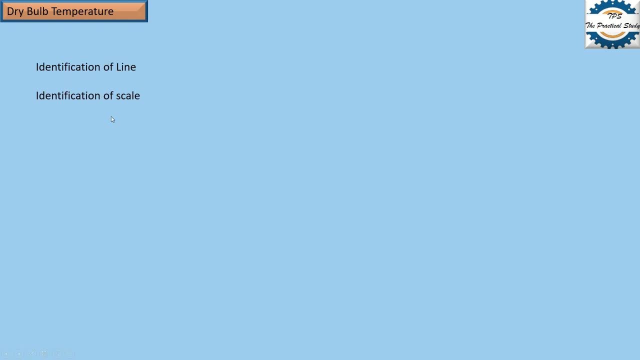 points, then this chart will be very easy for you. Suppose this is psychometric chart. let's draw dry bulb temperatures on this chart. This is the scale on horizontal axis or x axis for dry bulb temperature and it increases from left to right. So we will find out the scale of the parameter which is on horizontal axis. 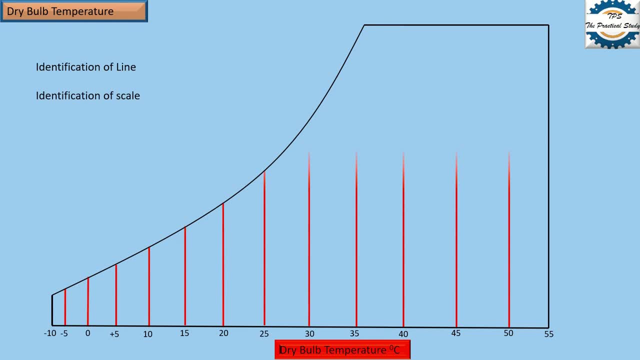 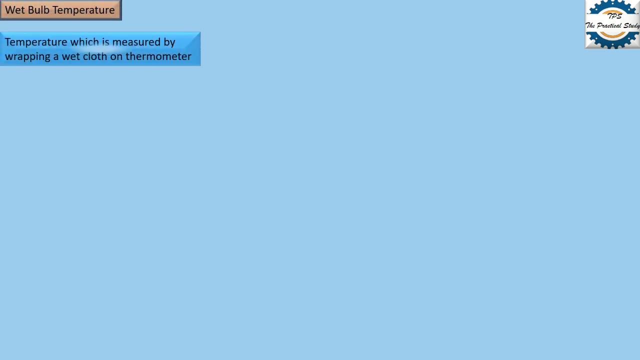 Now let's draw the lines of dry bulb temperature. These are the lines of dry bulb temperature on psychometric chart. I think dry bulb temperature is clear right now. Let's move to the next parameter: Wet bulb temperature. This is the temperature which is measured by wrapping a wet cloth on thermometer. 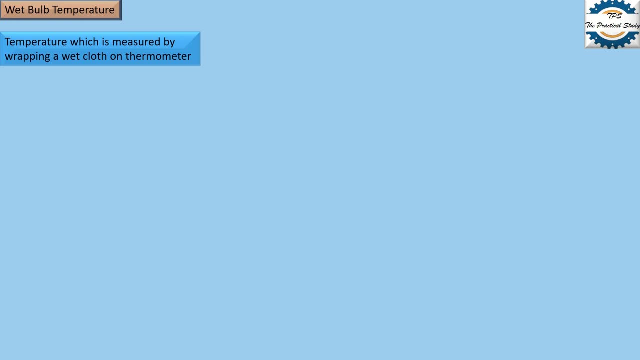 We have already made a video on this topic. Let's find out Its line position and its measuring scale on psychometric chart. This was the scale of dry bulb temperature, These are the lines of wet bulb temperature And here is its scale. 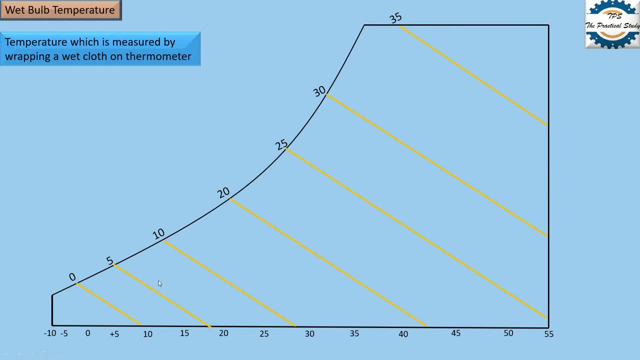 So wet bulb temperature lines are, as seems to be, inclined line around at the angle of 25 to 30 degree. These lines shows the wet bulb temperature, These lines show the wet bulb temperature, Wet bulb temperature line and this scale shows wet bulb measurement scale. 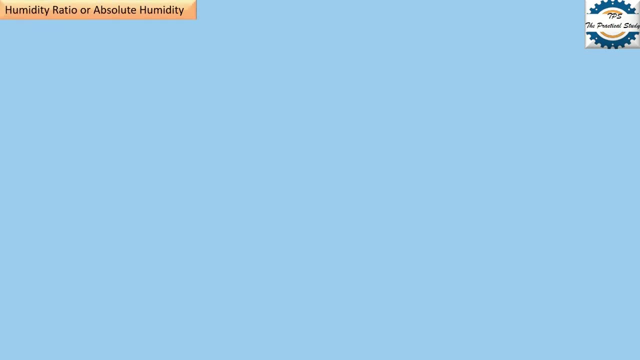 Let's move to the next parameter: Humidity ratio or absolute humidity. For example, if you have a 1 gram of air, then how much water is present in 1 gram of air? in grams, This is humidity ratio, Since in 1 gram of air the water quantity or water vapor's quantity is very much less. 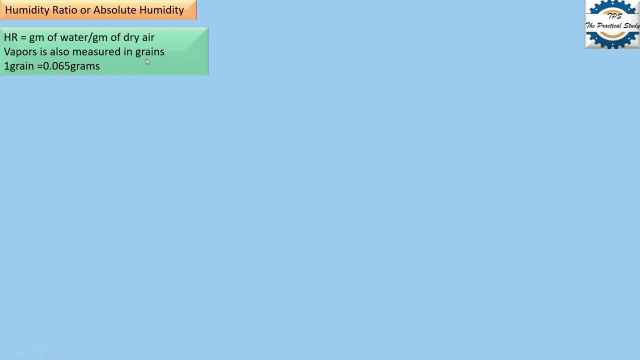 so vapor's is also measured in grain, which is the smallest unit of water vapor's quantity. One grain is equal to 0.065 grams. When you have anything in smallest quantity, then it is better to measure it on smallest scale. Let's draw it on psychometric chart. 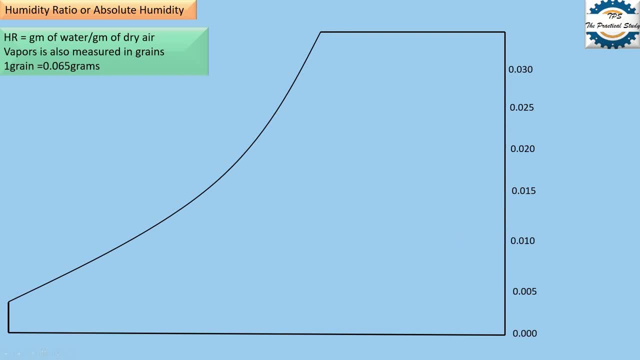 Humidity ratio scale is on the y axis, on vertical axis. Now let's draw its lines. Its lines are horizontal towards the wet bulb temperature line. I think this parameter is also clear. Let's move to the next parameter: Relative humidity. Relative humidity is the amount of water vapor's in form of percentage. 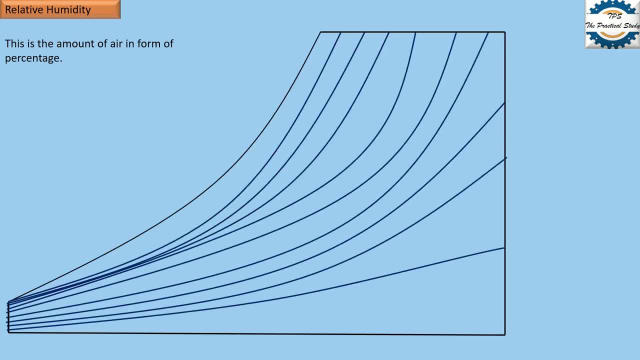 So this is psychometric chart And these are the relative humidity lines. And here is the relative humidity line And here is its scale. I think this parameter is also clear. Next move to the next parameter. Now, guys, one point: you need to notice that this is the saturation line, where the humidity 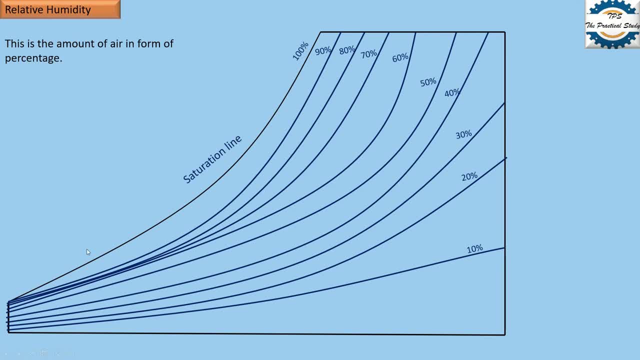 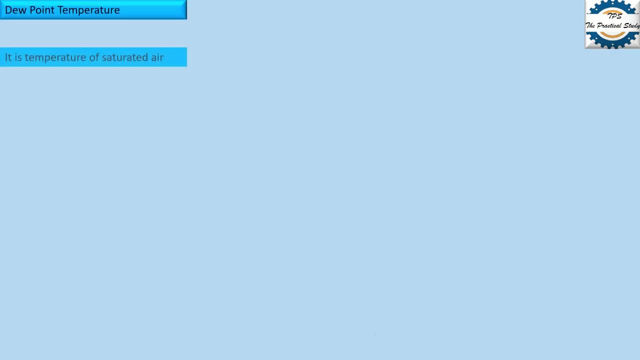 is 100%. That means air is fully saturated. Air is full of water vapor's and there is no more possibility for absorption of more water vapor's. Due point temperature. It is temperature of saturated air. What is saturated air, For example? this is air, and when it becomes full of water vapor's then it is called saturated. 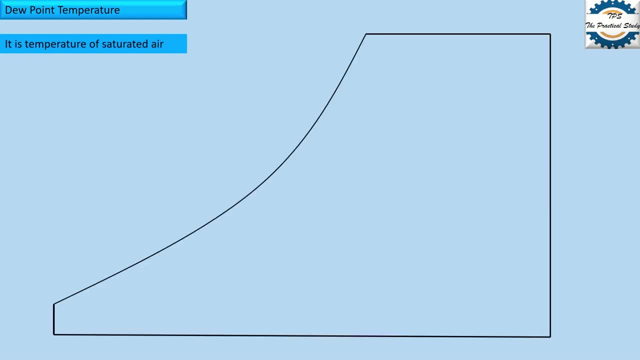 air. So the temperature of saturated air is called due point temperature. This is the scale of wet bulb temperature and it is also used for due point temperature scale Because this scale is This scale is Drawn on saturation line, As you can see that where the humidity is 100%, 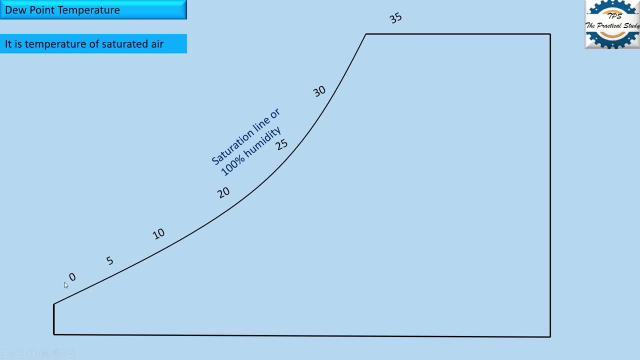 So this wet bulb temperature line and saturated line is used to measure the due point temperature. You, specifically the due point temperature lines, are seems not to be plotted on the psychometric chart. But how can you find the due point temperature? It is very simple. 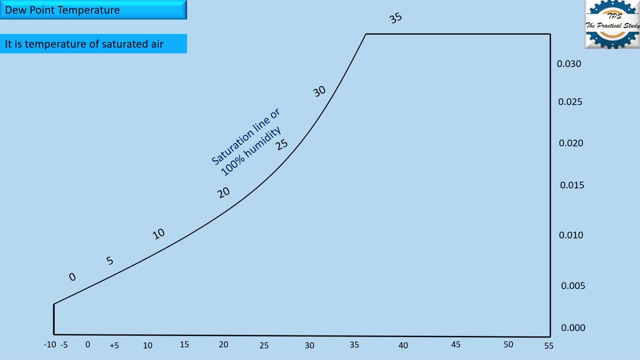 Let's suppose this is dry bulb temperature scale. This is humidity ratio scale. If these two parameters you have no None, then you can easily find out due point temperature. For example, you have dry bulb temperature 28 degree centigrade humidity ratio: 0.013. 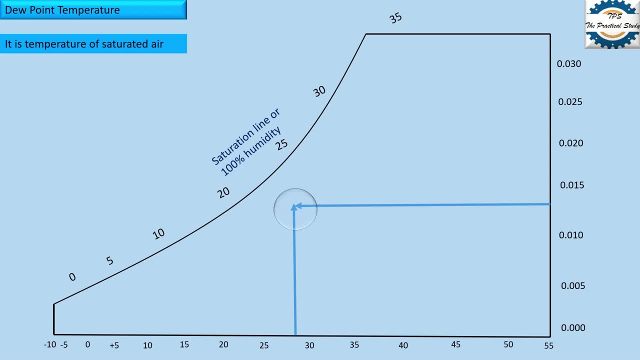 Then, at the point of intersection, you draw a horizontal line towards the wet bulb temperature line in order to find the due point temperature. I hope this is clear. Let's move to the next parameter: Specific volume. Specific volume And also enthalpy. 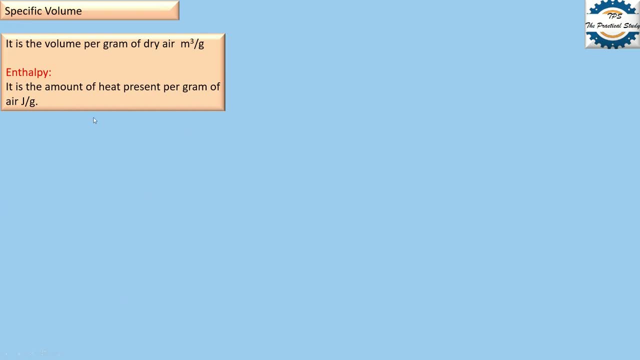 Specific volume and enthalpy we will discuss in single slide. Specific volume: it is the amount of, it is the volume of air in per unit gram of air. Its unit is meter cube per gram, or in other words you can say that if you have one gram, 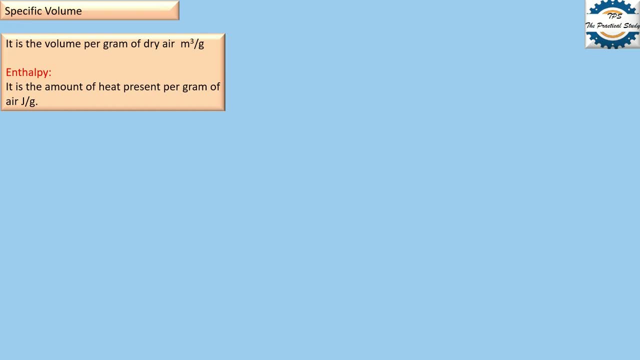 of air, then what is the volume of one gram of air? is specific volume And what is the enthalpy? If you have one gram Of air, then how much heat is present in one gram of air is enthalpy? Its unit is joule per gram. 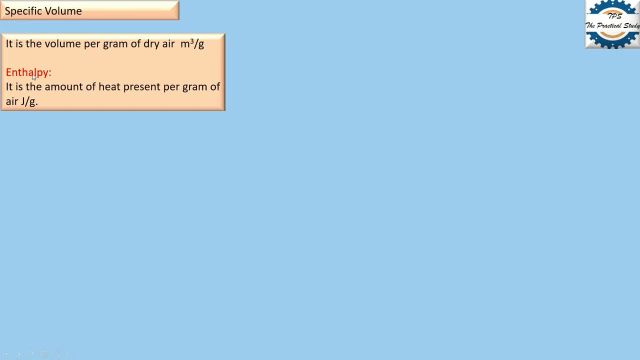 Now let's draw these two parameters on psychometric chart. This is wet bulb temperature lines. Why I have drawn it again? because the enthalpy lines are very much similar to wet bulb temperature line, but these lines are extended towards the enthalpy scale. 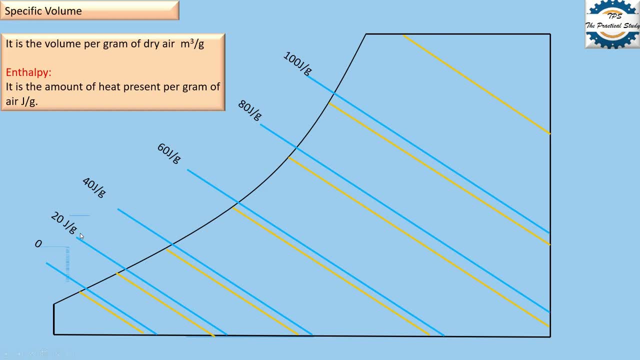 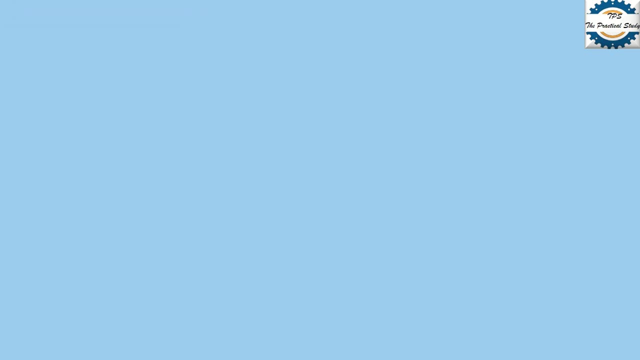 I think it's time to draw a complete psychometric chart. Suppose this is the psychometric chart. First we have drawn the scale of Dry bulb temperature, Then scale of humidity ratio, Then scale of enthalpy, Then scale of wet bulb temperature. 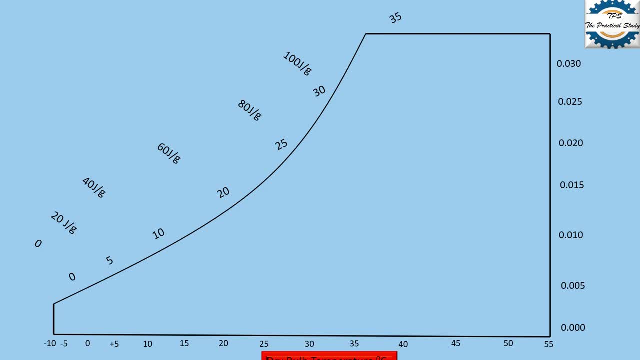 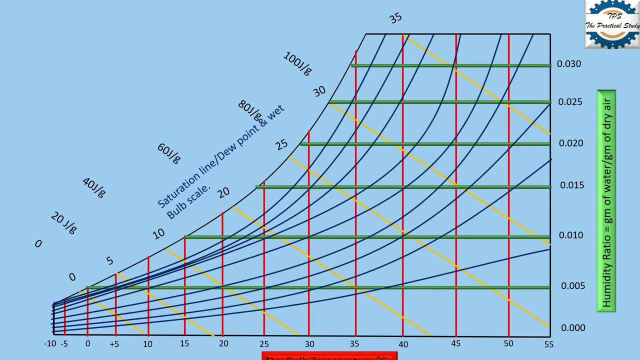 Saturation line, Dew point, temperature Scale. Now draw the dry bulb lines, Draw the wet bulb lines. Now draw the humidity ratio lines. Now draw the relative humidity lines And now draw the wet scale. Next, we have drawn all the Hebrew values. 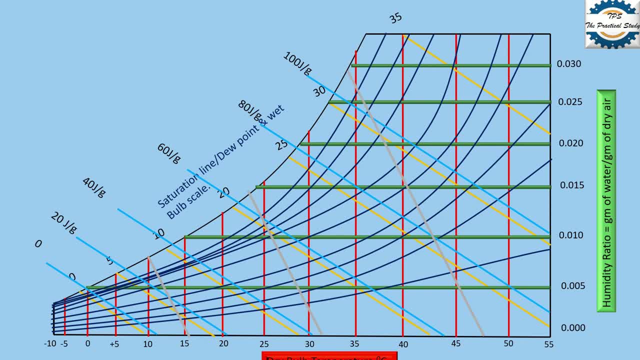 That is about 10.2.. enthalpy lines, or rather specific volume lines, this is a scale of specific volume and this is the scale of relative humidity. so this was that complex chart which we didn't discuss in earlier. I hope I tried to make it very clear to. 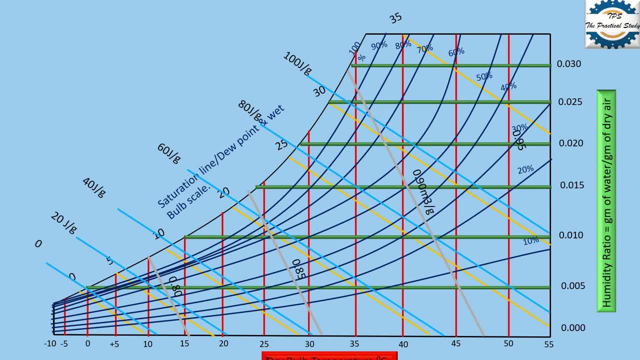 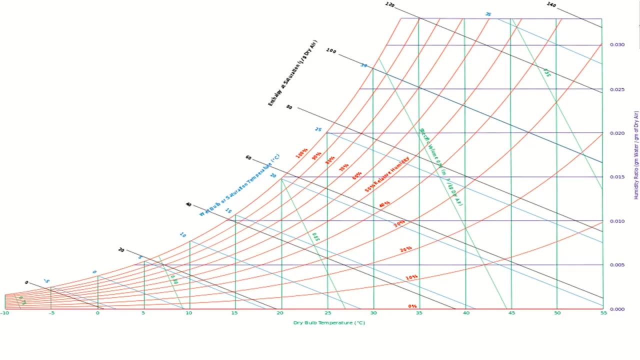 you. so it's time to solve a practical example that how we can calculate required parameters on psychometric chart. for calculation of parameters, I think, we move to professional chart. so in order to get the correct values, in order to use psychometric chart, you must have two parameters. if you have two, 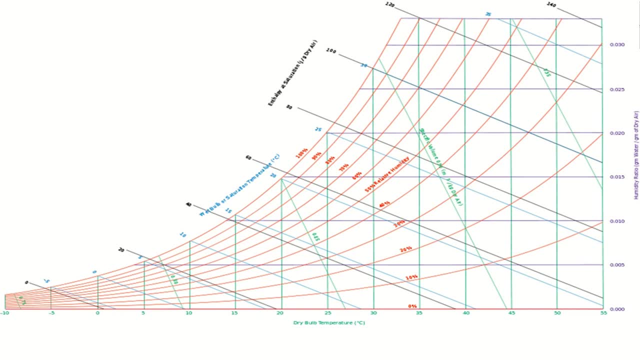 parameters and by the intersection of that two parameters you can find out all other parameters. how, for example, your dry bulb temperature is 30 degree centigrade, your wet bulb temperature is 25 degree centigrade, and you need to find relative humidity, specific humidity, dew point, temperature, specific volume. 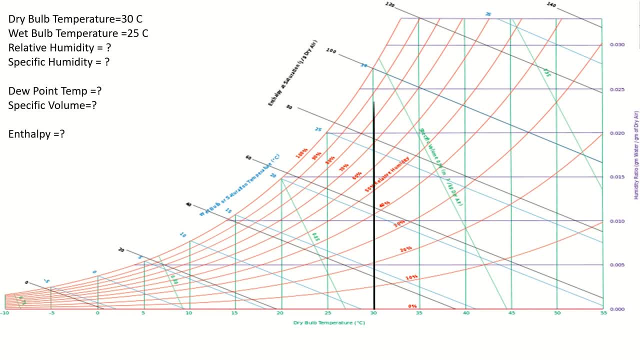 enthalpy. so what you have to do, first you need to draw your first given parameter and then second given parameter, once again, dry bulb temperature: 30 degree centigrade. so I draw the line on 30 degree centigrade parallel to the line of dry bulb temperature. remember one thing: 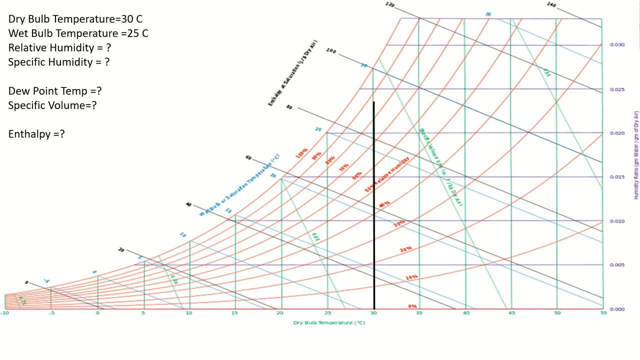 whatever parameter you have drawn, it should be parallel to that parameter. for example, wet bulb temperature: 25 degree centigrade, and these are the lines of wet bulb. so my point is also on 25, so my line would be parallel to the that 25 line. so then we find the point of 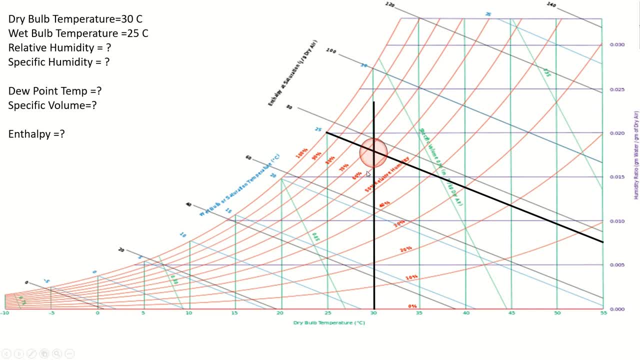 intersection. this is my point of intersection. now, guys, what you have to do, you have to draw a line from the point of intersection to the point of required parameter scale, but your line should be parallel to the required parameter scale. it once again whenever you want to find out a parameter on: 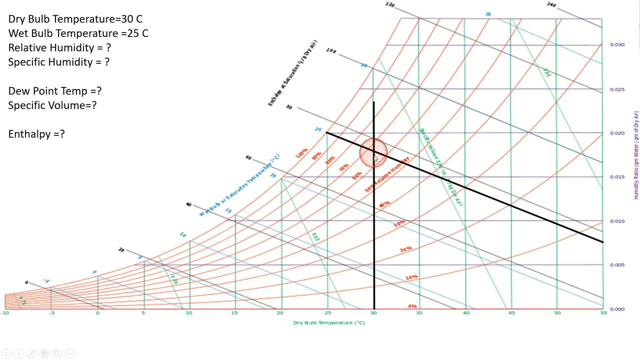 psychometric chart you need to draw a line parallel to that required parameter line till the scale of required parameter, for example relative humidity. my intersection point is between 60 percent humidity line and 70 percent humidity line. if I draw a line parallel to these lines then 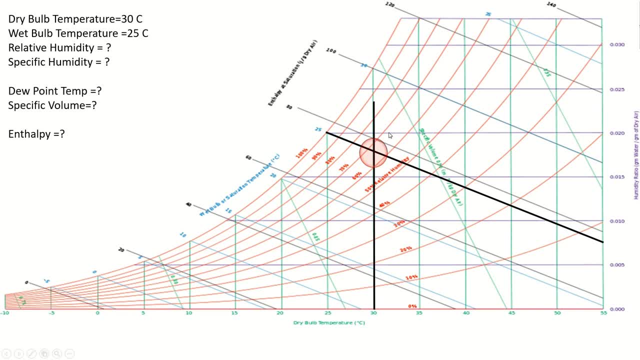 you will see a line parallel to the line of the required parameter scale and it will be nearest to 70% line. so my relative humidity is around 68%. Specific humidity or relative humidity: my specific humidity lines are horizontal, so when I draw a horizontal line, 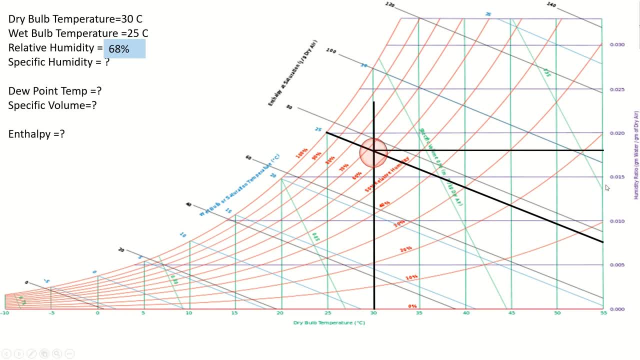 parallel to these lines, to the scale of humidity ratio, so I can get specific humidity. My specific humidity point is between 0.015 and 0.020, but it is nearest to 0.020, so my value is 0.018.. For dew point temperature line, as we have already,